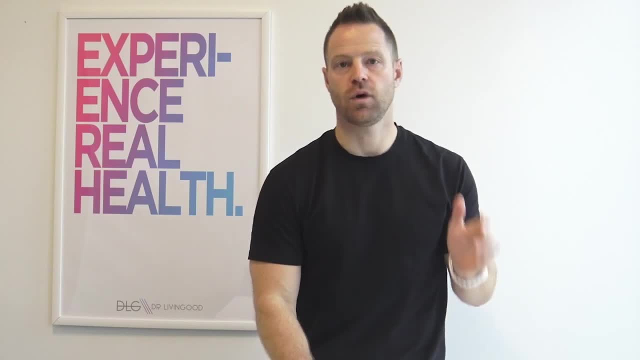 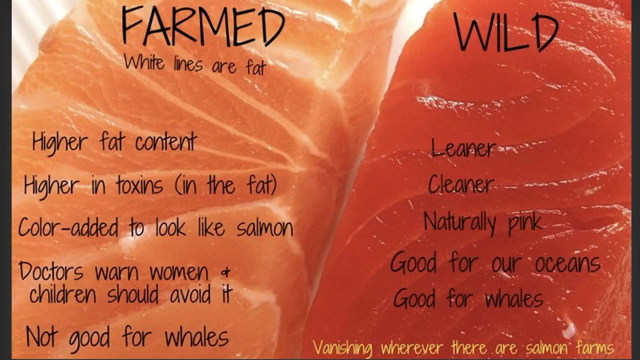 from. It comes from their diet. Remember: you are not what you eat, You're what you eat. ate. Try to say that one a couple of times fast. The color is then added to make it orange, Otherwise that farm-raised salmon ends up gray. I'm telling the truth. 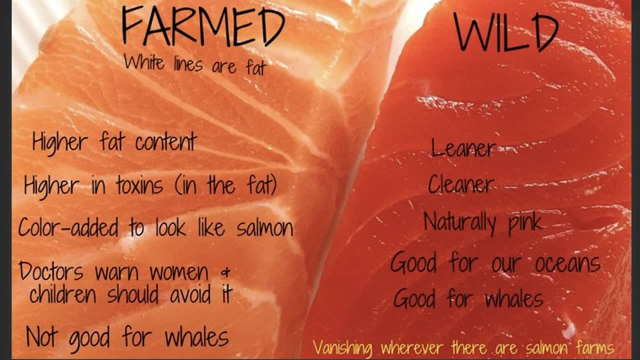 You've laid one of those farm-raised salmon open, You would find a whiter, grayish tint to their meat. Doctors warn that women- children, should avoid it, especially this type, And it's really hard on the whale population. honestly, Wherever there's these large farms of salmon, well they're. 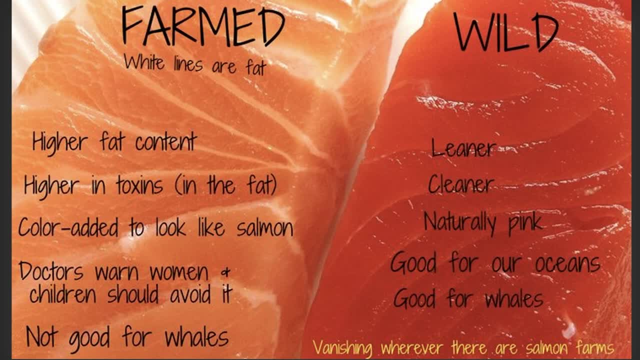 consuming all of the food in the area and then they're feeding them pellets and synthetic food, and so not good for the whale population From a wild standpoint. you're going to get much leaner, much cleaner, naturally pink, And the pinkness comes primarily from their diet. They're 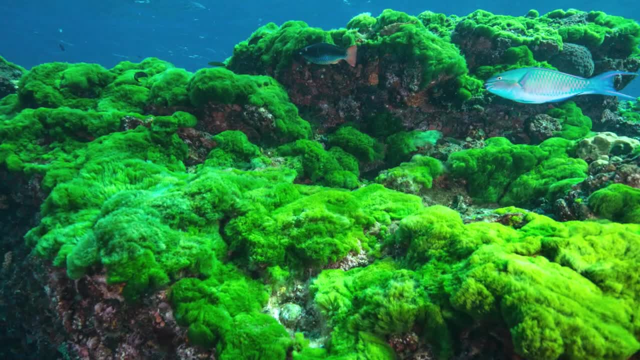 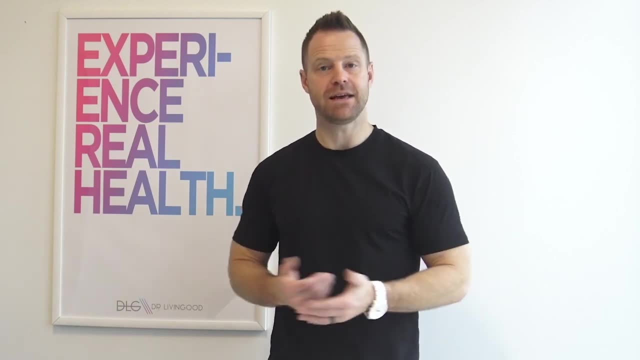 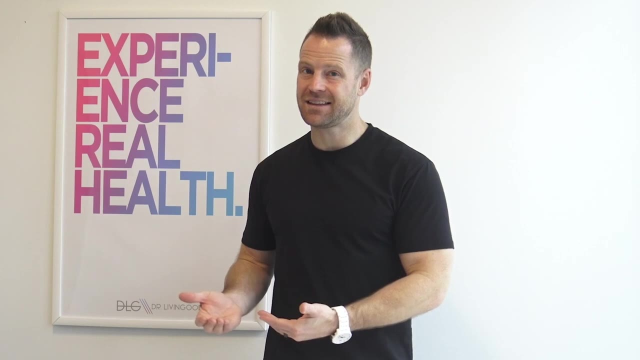 going to feed on crustaceans and shrimp and algae that are actually full of the needed vitamins and astaxanthins that are needed to actually naturally make them that pink color. So a salmon in nature feeds off the proper foods to give it the pinkness. A salmon in a farm doesn't get those. 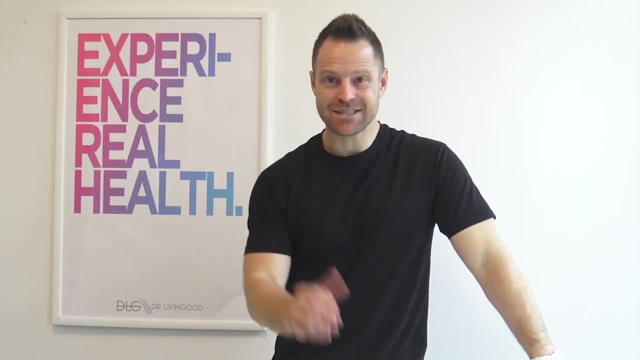 or do they? They do They feed them synthetically. So I actually did some research into what farm-raised salmons are fed. Look at this: You're not what you eat. You're what you eat- ate. This is a whole. 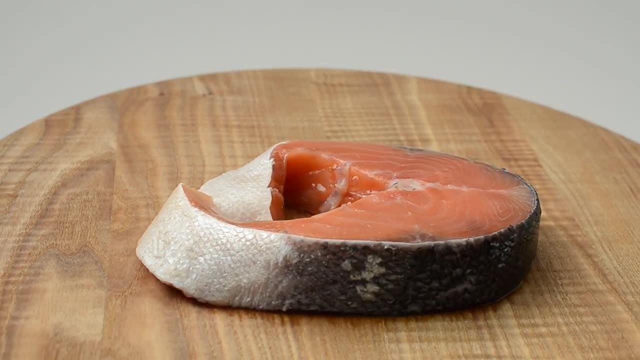 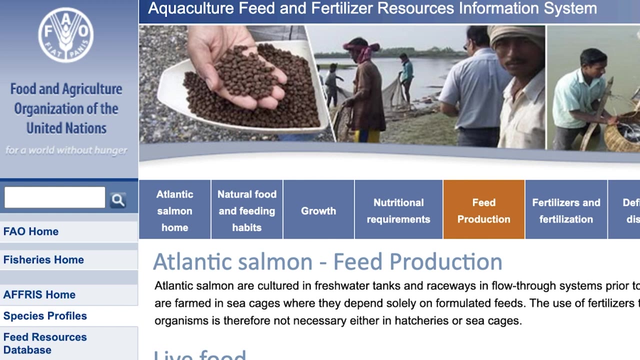 nother level when you start looking at what exactly is the meat you're eating. What were they fed? Because whatever they were fed is going to end up and trickle down into you. Check this out. This is the Food and Agricultural Organization of the United Nations, and they are specifically. 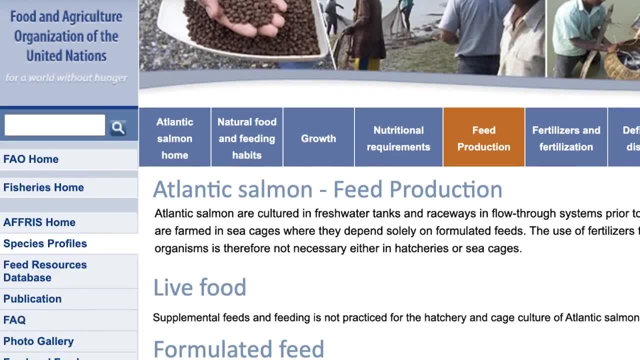 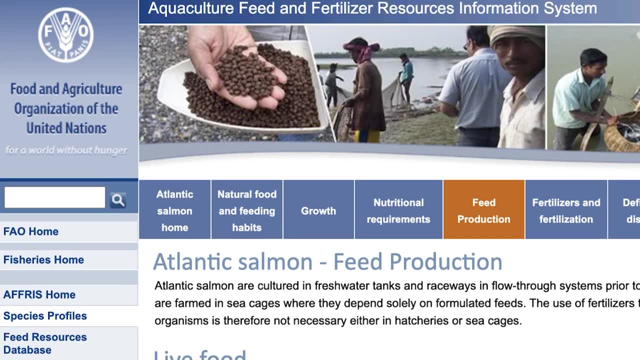 looking at feed production and food formulas for salmon. You can go on this website, right? So this is a government agency, right? That is controlling this of what they are fed, And you can see these fish operations. I would just hate to go on site to some of these what they look like, but let's go. 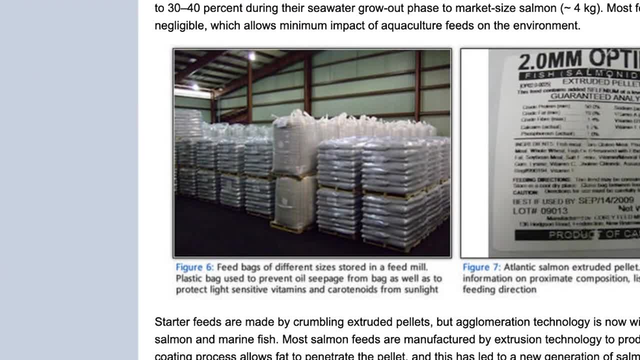 down. So here's like the palates of the food, right, And like just what I teach you with food. it's like, well, don't read the front of it, Don't read the nutrition facts. Let's actually go to the 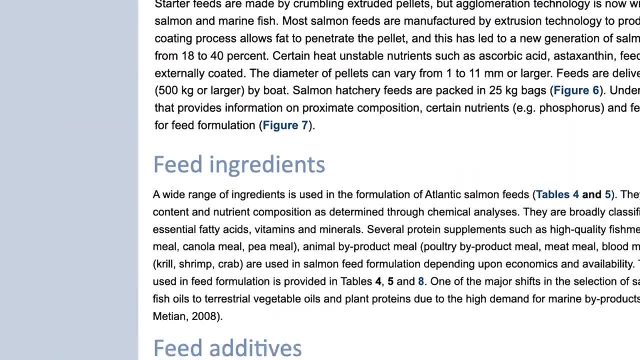 ingredient label. So we keep going down. Here's the feed ingredients They actually give it And I thought, wow, we should probably break this down a little bit And there's a lot to this. but there's additives and there's actual ingredients. So we're going to go down here and we're going to look at. 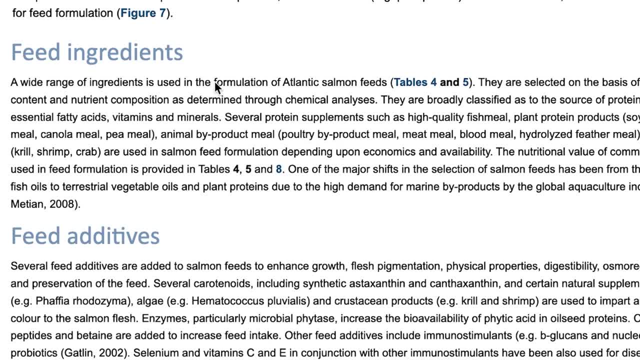 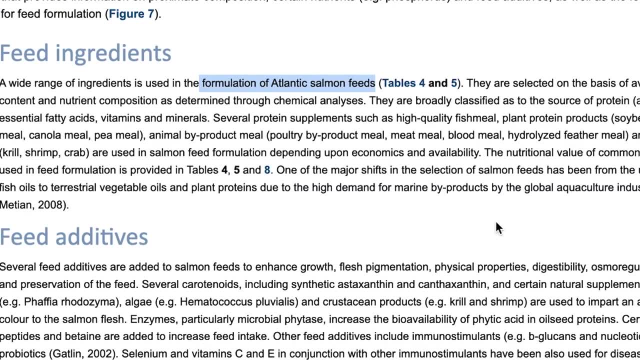 additives and there's actual ingredients. So, as we start to look through the formulation of Atlantic salmon feeds, they're selected on a basis of available energy and content and nutrient composition as determined through chemical analysis. So you're going to have some protein in there. You're going to have some fatty acids in there, You're going to have some. 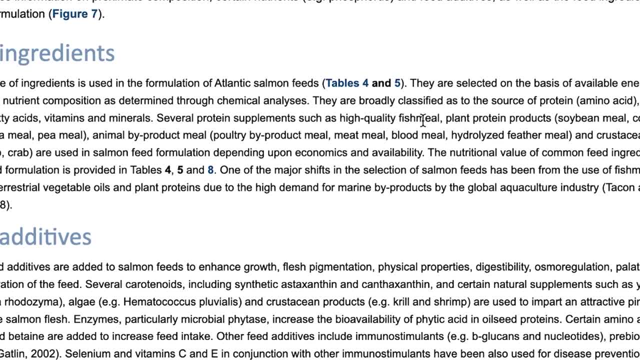 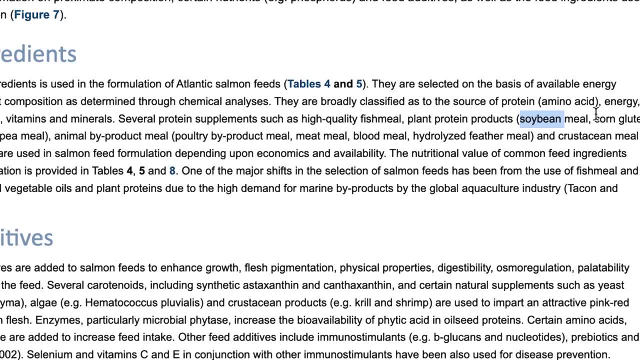 vitamins and minerals, but they're synthetically putting this together as a fish meal So they might put soy. Now we're looking at genetically modified organisms ending up in your fish. So now it's genetically modified, We're going to get corn. same criteria. 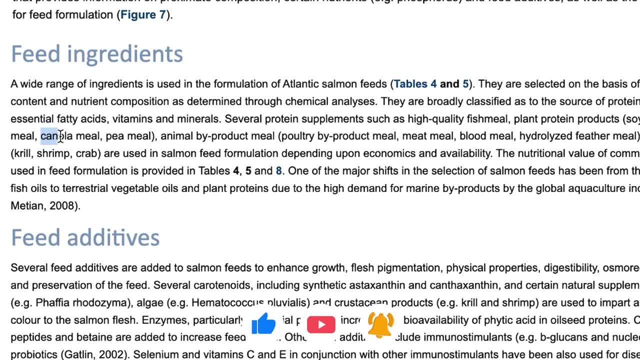 If you've watched any of my other videos, you also know my stance on canola. There's actually canola meal, highly inflammatory, chemical, laced hexane, laced seed oil. Then we have peat. No problems there. typically There's animal byproducts that they're fed, whether it's a 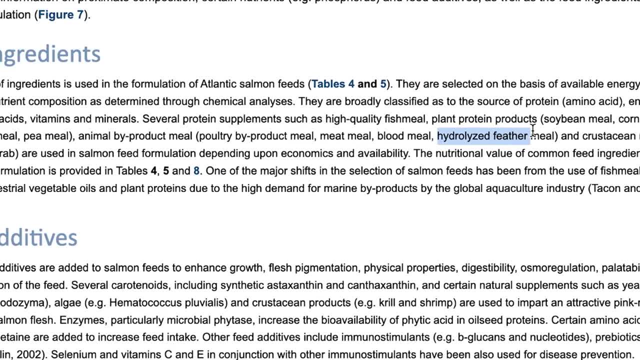 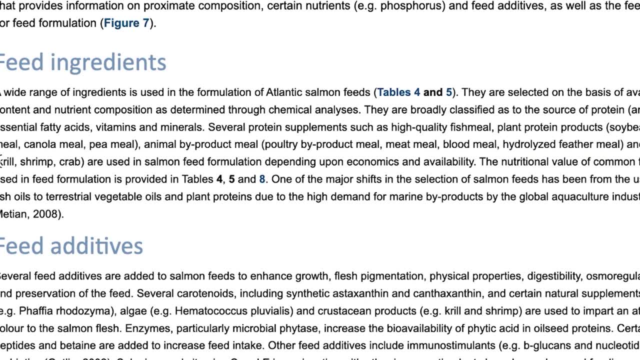 meat meal, a blood meal, a hydrolyzed feather meal- grinding up feathers, using parts from other animals to feed these- And then there's the actual crustacean meal, which is more so what they should be eating: Krill, shrimp, crab. This is what gives them their pinkness. 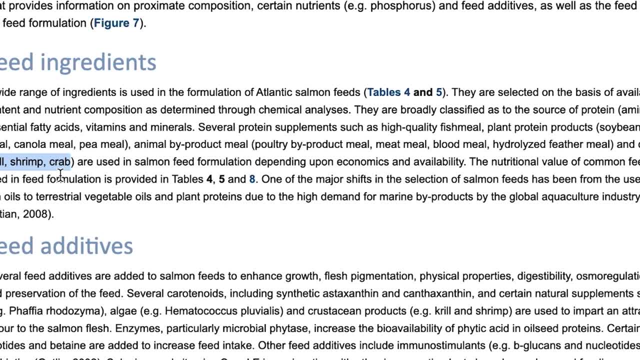 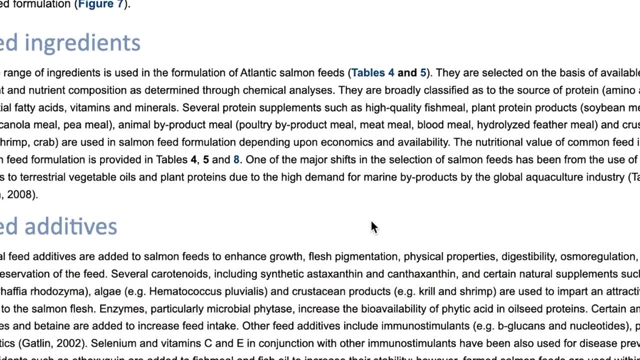 So I don't have much problem with those. That's what it should be, but that's expensive, So they don't do it, depending on economics, right? We're seeing it right there. So let's move down. What do they add to this thing? To enhance the growth, the flesh pigmentation, pinkness and physical. 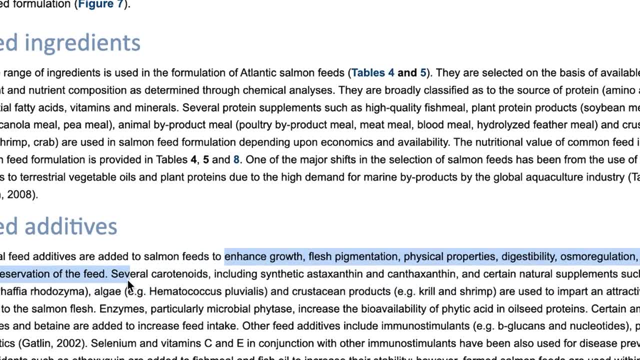 properties, digestibility, all of these right. Preservation of the feed. Several things are added. Number one: they use carotenoids. Now, that's a vitamin A, Normally not a problem, but these are synthetic forms that they're putting in to make it pink, including synthetic astaxanthin. I don't 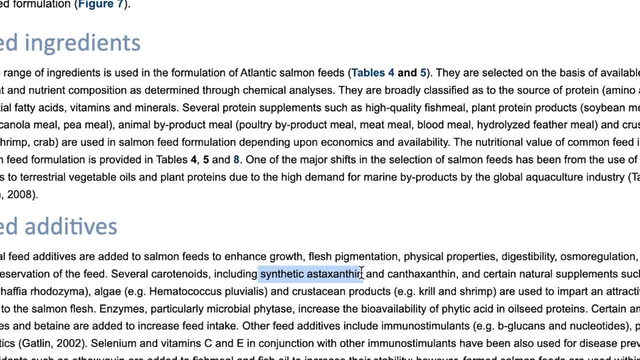 have a problem with true krill oil astaxanthin coming from the pinkness of a shrimp or a krill or an algae or a flamingo- right, We're not going to get it from flamingos, but they have this natural astaxanthin, which is an incredible antioxidant if taken in the right amount. But this synthetic 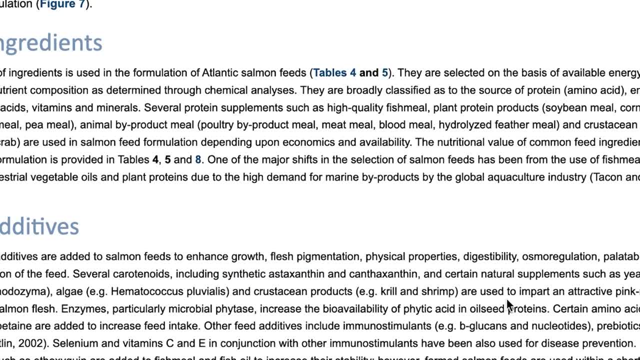 kind, not the case. More on that in a moment. This is what is used to impart the attractive pink and redness, So they put it right on here. This is developed in the 40s, 50s and 60s to. 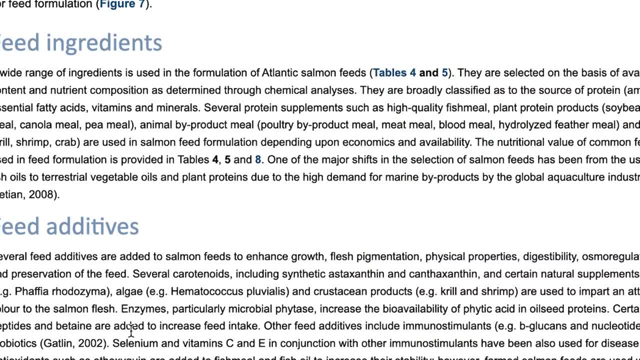 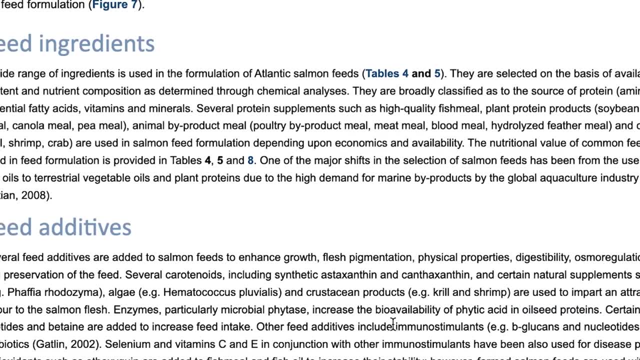 really start to do this so that when it hits your sushi plate you see that pinkness, that bright pinkness. You know that is synthetic astaxanthin. We're getting more bad oil seed proteins that are added to it. Immunostimulants are put in, stimulating the immune system, And there is 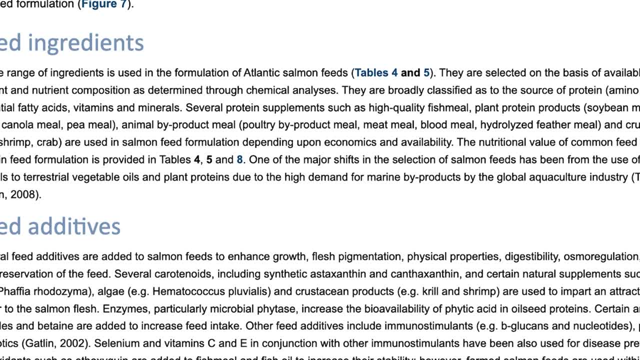 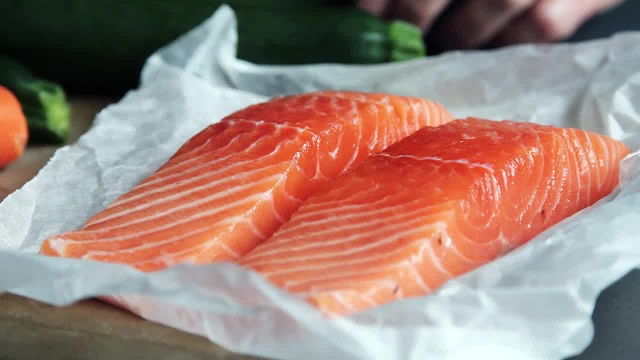 some nutrients added to it, thank God, And then we use gelatins and things to hold it together, starches and other chemicals. So this is what's ending up in the actual farm-raised salmon That's going to end up in you if you're eating that meat. That pink colorization, though, comes. 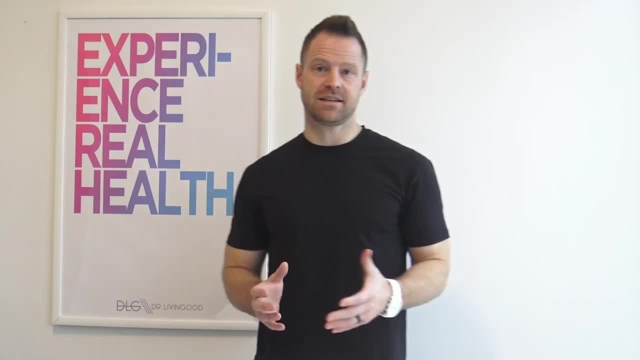 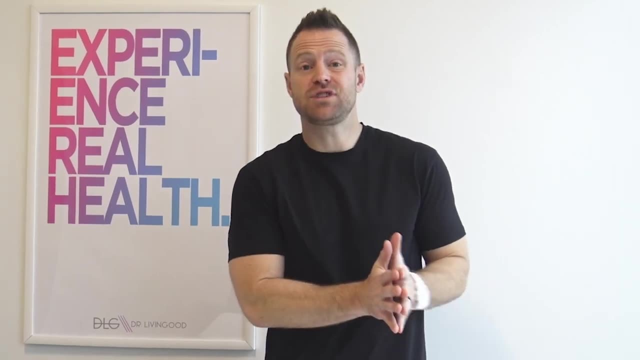 from that synthetic astaxanthin. The issue with the astaxanthin is made from petrochemicals. Not a single human trial has been done on the safety of that And we've been using it for 70 years in the fish industry because you'll pay a dollar more for the pinkness of the meat And if 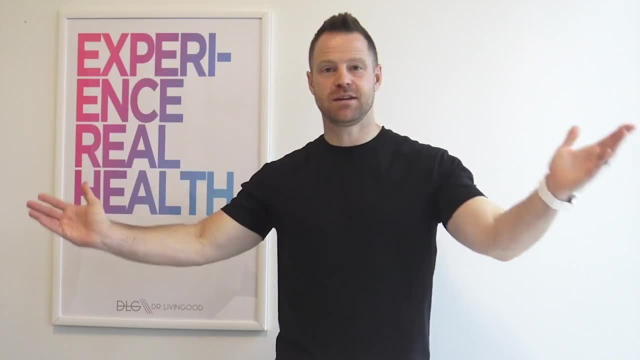 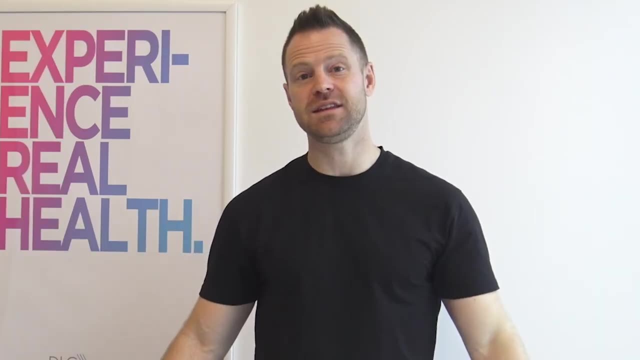 salmon goes gray because it's raised on a farm. it's going to blend in with every other meat and it won't stand out and you won't buy it. So salmon farmers have literally admitted this, knowing. I wish we didn't have to feed them a more expensive synthetic astaxanthin. 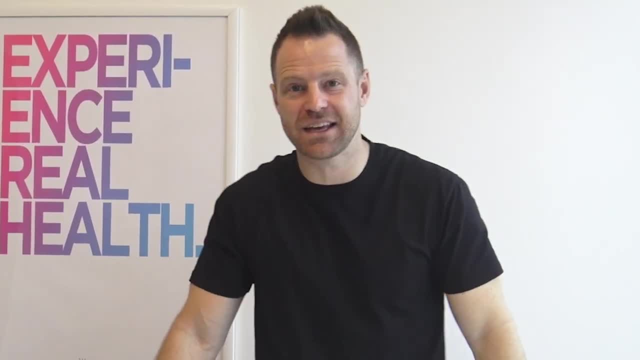 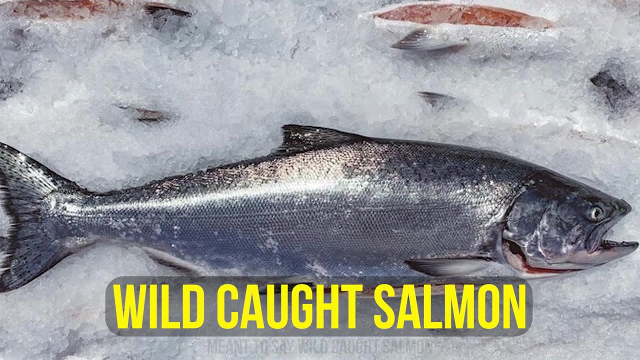 but we have to because they need the coloring. It's just part of the game that they're playing. So point being: look for farm-raised salmon. Way better nutrient content, true coloring with true antioxidants, way less fattiness, way less chemicals going to you and. 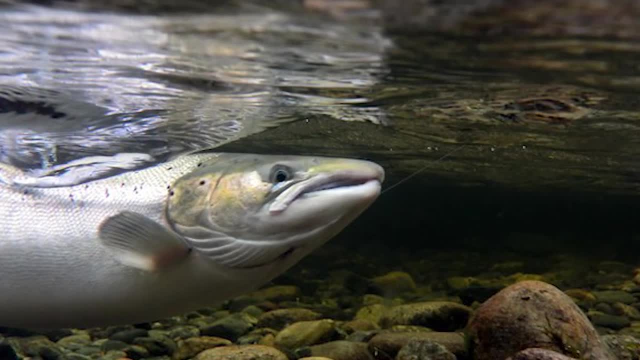 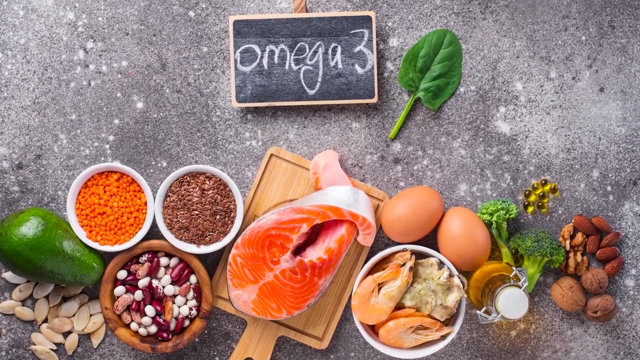 your family's body. Salmon should be eating little algae, krill, shrimp, small fish to get those colorings. And if you're looking for the omega-3 benefits, you're looking for the anti-inflammatory benefits of salmon, which is the reason why a lot of people are going to be eating it. 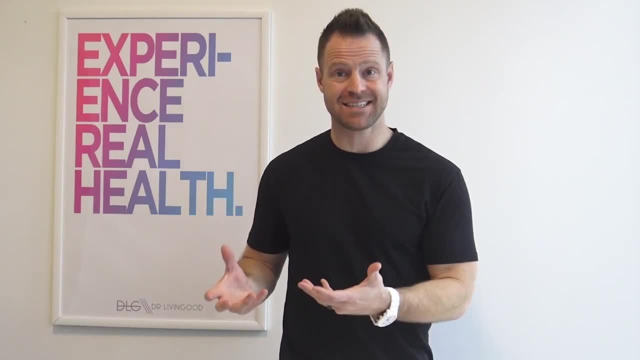 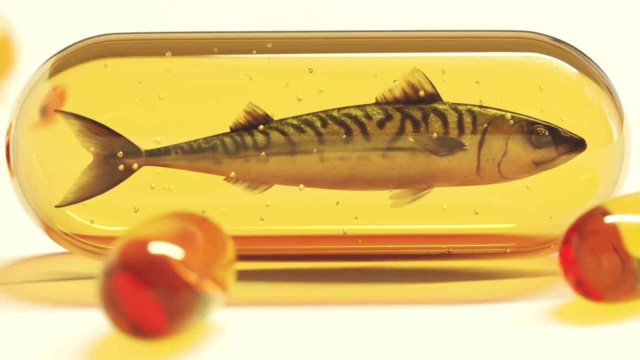 you can supplement with that. I use an omega that's sourced from Atlantic seas in very fresh, controlled waters, where you can get those small fish and then extract the omega-3, protect it, use antioxidants, So there's nothing synthetic involved with it. when you're looking at wild, 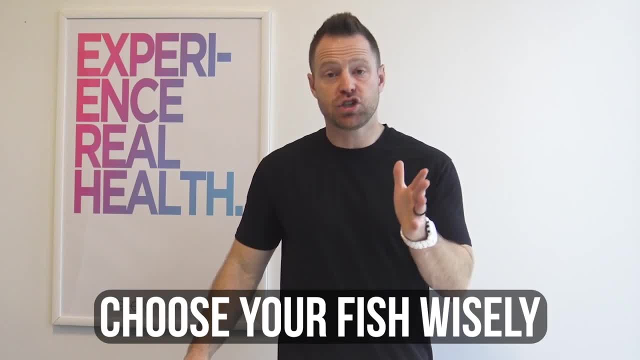 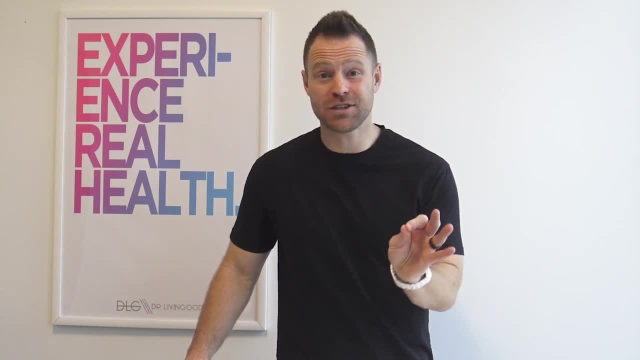 caught fish and then get the benefit of it. So there's a link for that below. but choose your fish wisely. Focus on wild caught, hold that standard and don't worry too much about only getting a pink fish, because chances are it could be synthetic anyway and it's just a. 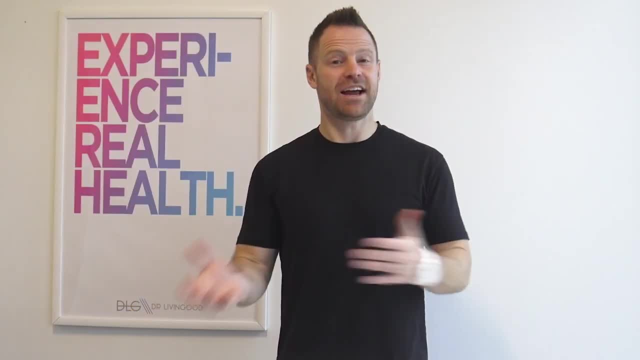 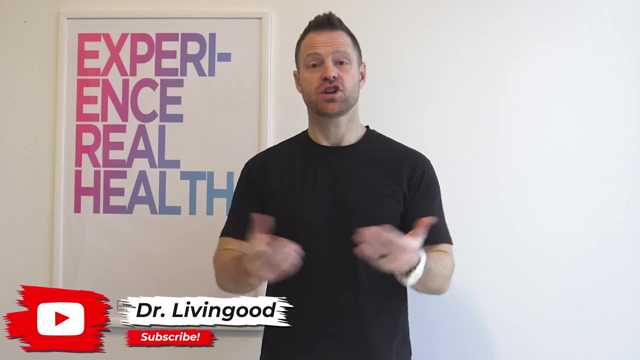 deception. Look for high quality fish, wild caught, to get your anti-inflammatories in Need. more help shopping for your meats, because the same thing is going to apply for chicken and beef, let alone fish. Come to the grocery store with me. I created a video where I actually